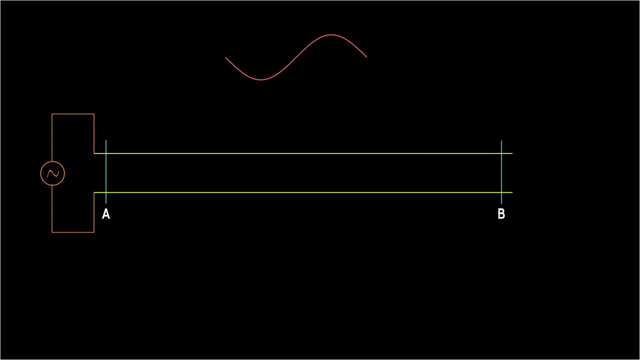 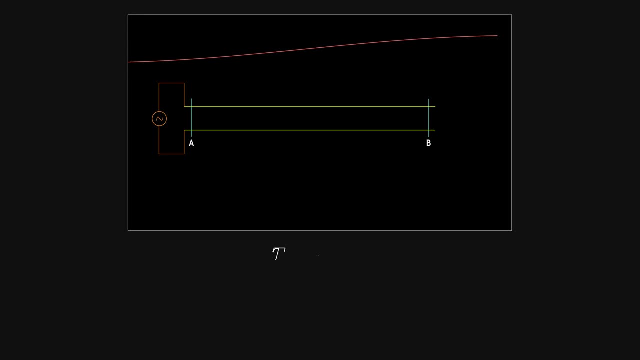 voltage difference between any two points on a line due to the finiteness of the speed of the wave. We can minimize that difference in voltage by decreasing the wave frequency. In other words, the higher the wave period with respect to transit time, the less would. 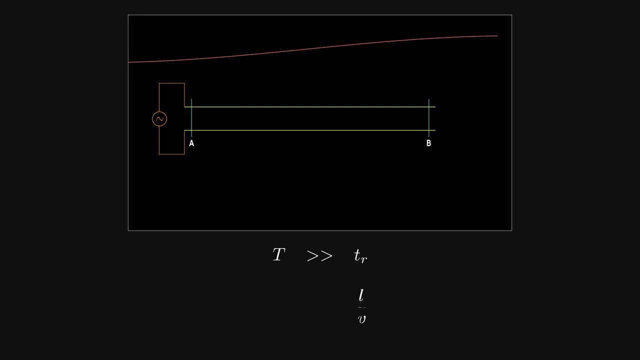 be the voltage difference. Transit time is equal to the distance traveled by the wave over propagation speed, while the period is equal to one over frequency. Hence, to minimize the voltage difference between point A and B on a wire, the length of the wire between point A and B must be very small compared to the wavelength. This concept 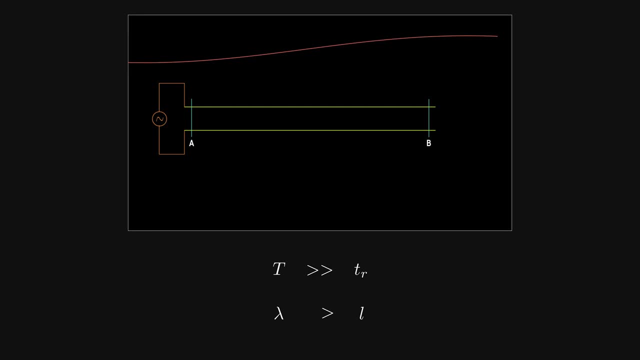 is applied to any electrical component. If the length of the component is large compared to the wavelength of the signal, then we can't ignore the transit time effect. To make Kirchhoff laws valid we must meet the conditions. The circuit element must be so small compared. 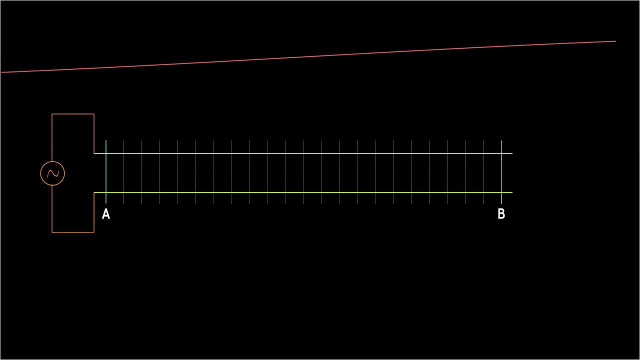 to the wavelength of the signal. If we divide this wire into smaller and smaller sections so that each section is too small compared to the wavelength, the transit time effect would be negligible over each section. so we can apply low frequency circuit analysis. That wire is called transmission line, a path. 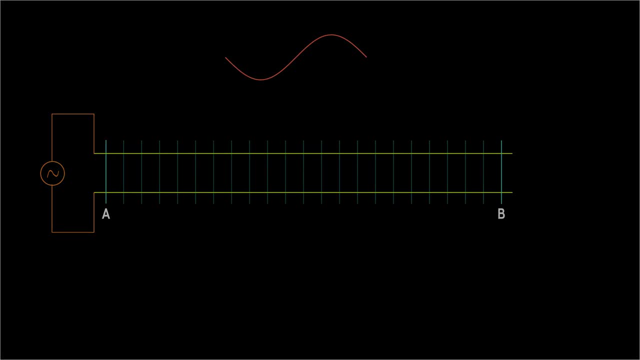 carrying electrical energy from source to load. Consider a transatlantic cable running from the US to the Great Britain, a good example of uniform two-line transmission line. If we short the other end and measure the input impedance, it looks like a big inductor. 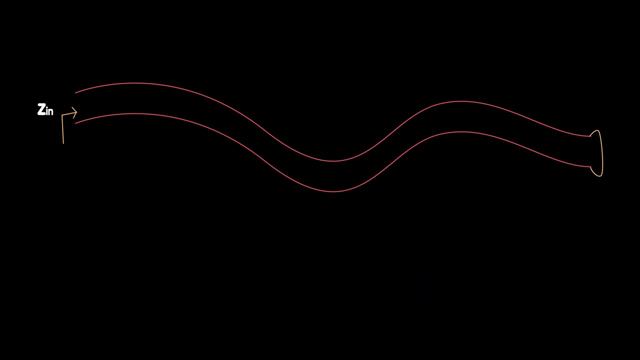 with a series resistor modeling the wire losses. Similarly, if we leave the other end open, the input impedance will look like a substantial shunt capacitor: two very big conductors separated by the electric Due to the conductivity of the shields, and the seawater. there is also 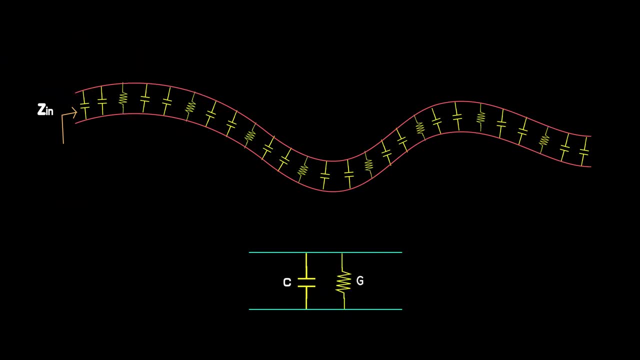 a shunt conductance associated with the cable, even when left open, Since the distance is too large. even at very low frequencies, the signal wavelength would be too small compared to the wire and the delay would be significant. So how do signals propagate through this cable? Well, each transmission line, as we just see. 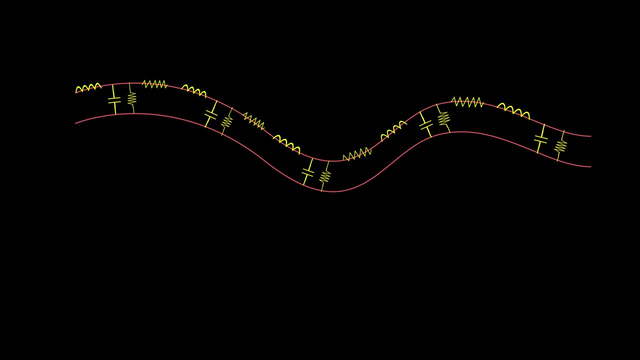 is composed of series inductance and resistance and parallel capacitance and conductance. Let's model the cable by them, then analyze the circuit, In other words lumping the total inductance, capacitance, resistance and conductance along the wire into either a series or a series. 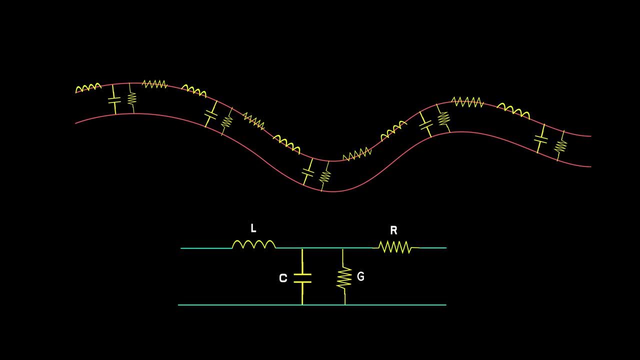 Here we have idealized concentrated components with infinitesimal dimensions and connecting between them with perfect conductors. This is known as the lumped element model. Using the lumped element model here gives us a completely wrong answer. Even at very low frequencies, the large series inductance would act as an open circuit, whereas the large shunt capacitance 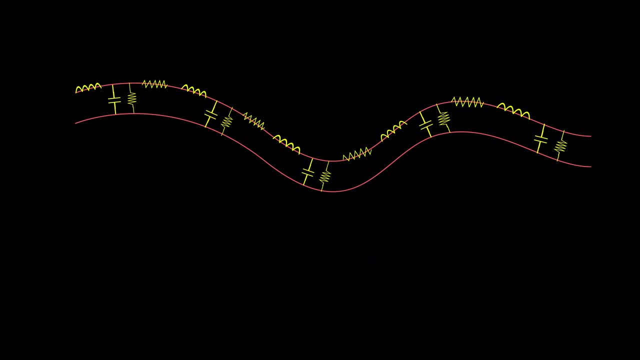 would make the wire a short circuit. For the lumped element model to be valid, the signal wavelength must be equal to the length of the cable. The signal wavelength must be very large compared to the circuit element. We can divide the total series and shunt impedances. 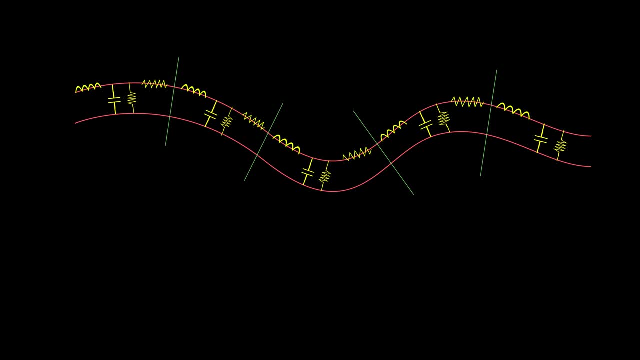 into smaller and smaller sections of very small dimensions compared to the wavelength. Let's ignore the losses for the time being, so that we can remove the series resistance and the parallel conductance from the model. And here comes the problem: For one centimeter long section we would need more than 500. 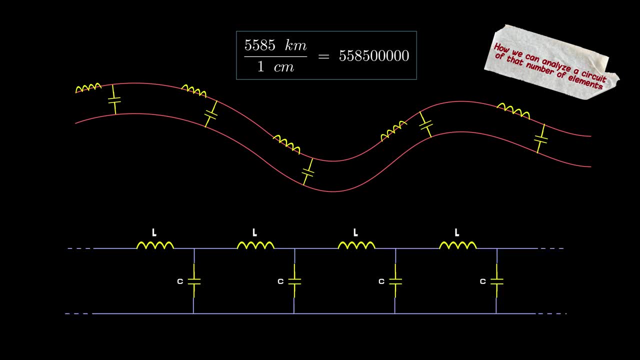 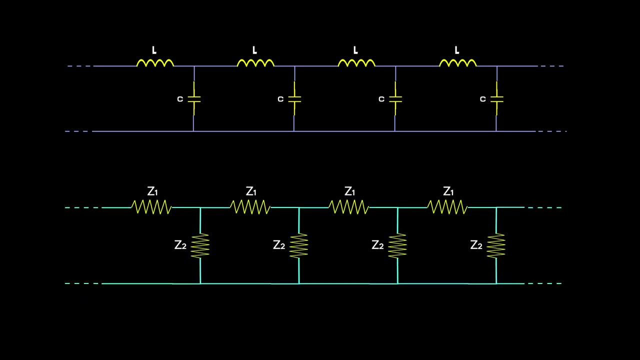 million inductors and capacitors. Even the most efficient simulator running on the most powerful computer can deal with that. So how did people solve this problem when the first transatlantic cable was laid out in 1857? Well, have you heard about infinite ladder networks before? This model is an infinite. 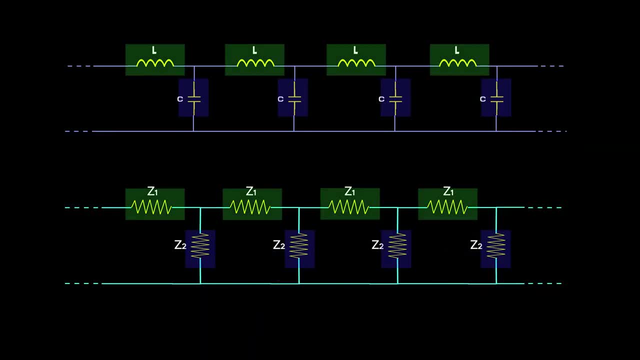 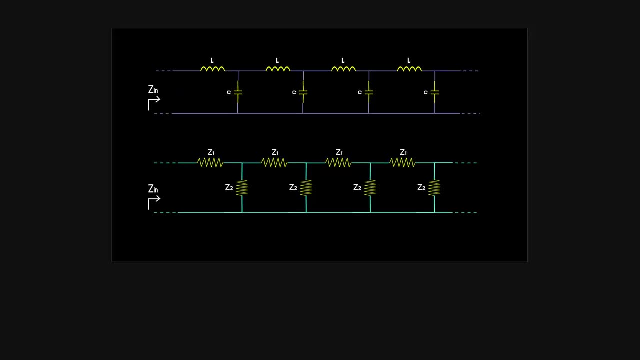 ladder network, with Z one and Z two being the impedances of inductors and capacitors respectively. Using the input impedance equation of the infinite ladder network, then the input impedance of such a cable is having that form. Since each section is on its own unit, the 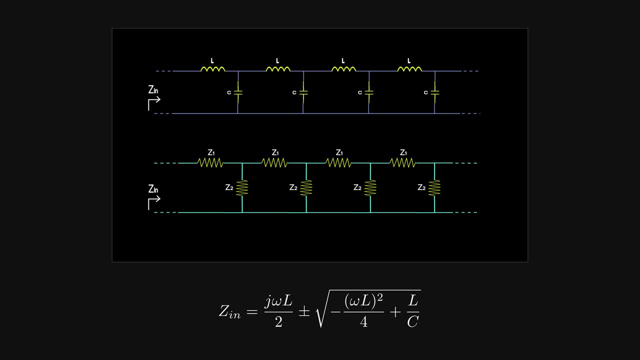 input impedance of each section is being controlled by the computer. Instead of using the input impedance equation of a cable, a cable is being controlled by a module. This is because the one centimeter long inductors and capacitors are too small and can be neglected making the input. 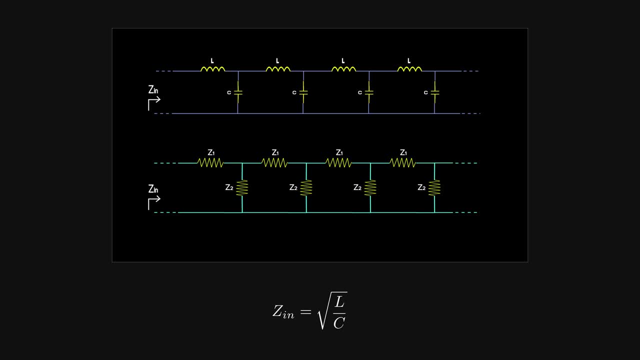 impedance equal to the square root of L over C. Observe that if we choose to terminate the ladder network with an impedance of Zn, then the input impedance remains the same. The behavior of a finite ladder section terminated with Zn is indistinguishable from that of the infinite. 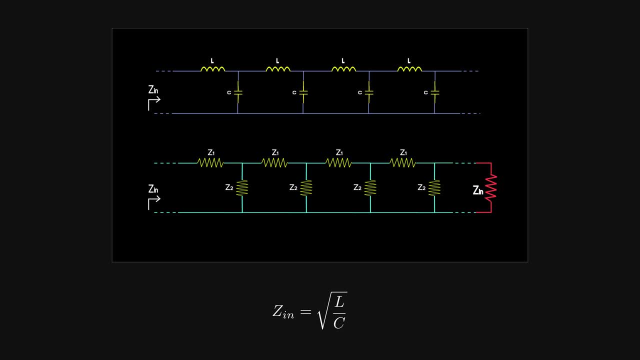 network. So for a lossless transmission line, the voltage wave will see a real impedance while traveling through the wire. This impedance is known as characteristic impedance. If the line is terminated with L of that impedance, the characteristic impedance would not change. Now we started by lossless elements, inductors and capacitors. 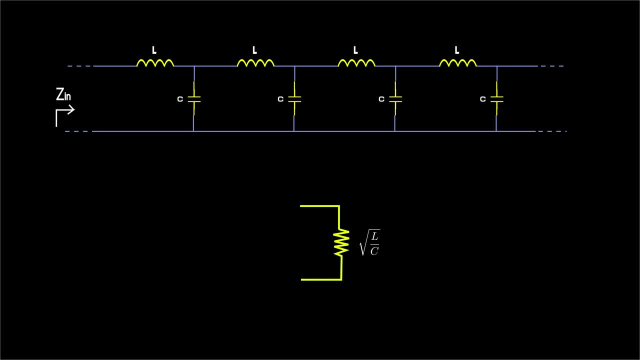 and end up with real impedance. Does that mean that the lossless transmission line dissipate energy? Actually not. The circuit is made up of lossless components. We have two scenarios here. If the line is infinite, the signal will travel through it indefinitely. 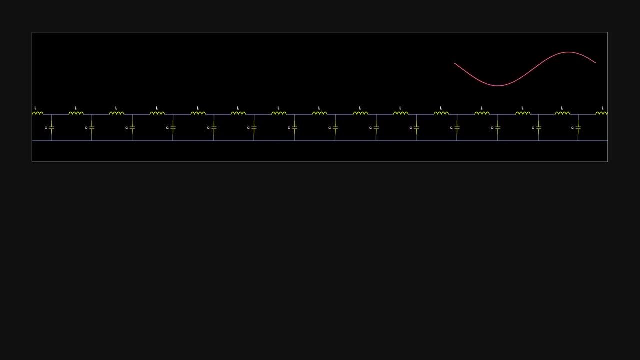 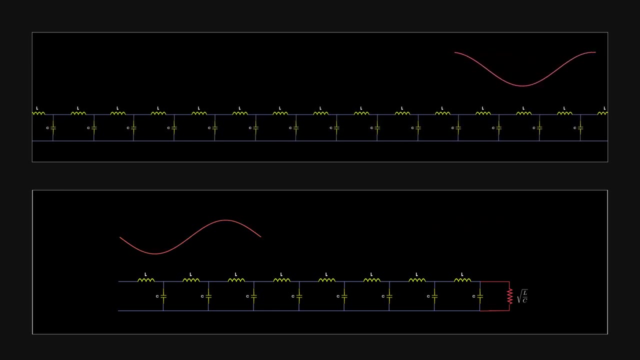 It is dissipated. from the generator perspective, If the line is terminated by resistance equal to the characteristic impedance, the signal travels through the wire and gets dissipated in the load. In both cases, the generator feels injecting the signal to resistance equal to the characteristic impedance. So far, so good. 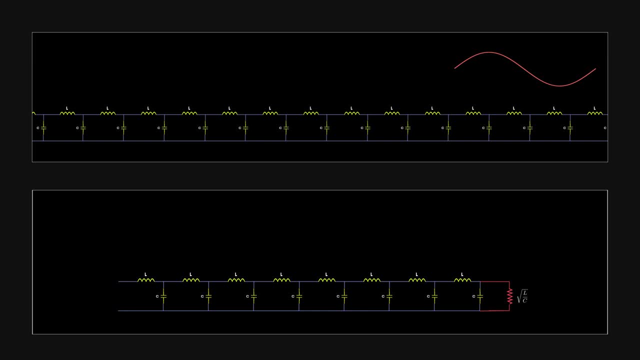 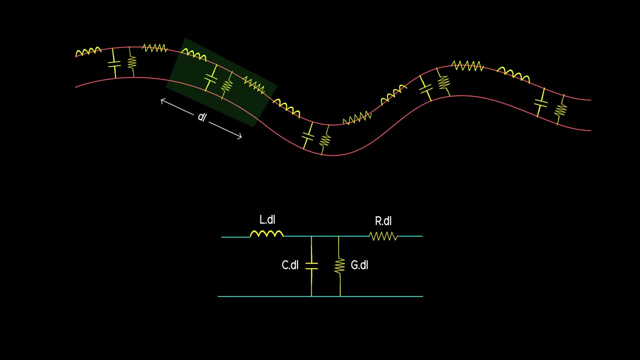 But how the injected signal itself propagates through the line. Now to answer that question, let's analyze one section from the line. Even at very high frequencies, the signal wavelength would be very large compared to the section dimensions. Hence the Lampt element model is valid and Kirchhoff laws can be applied. 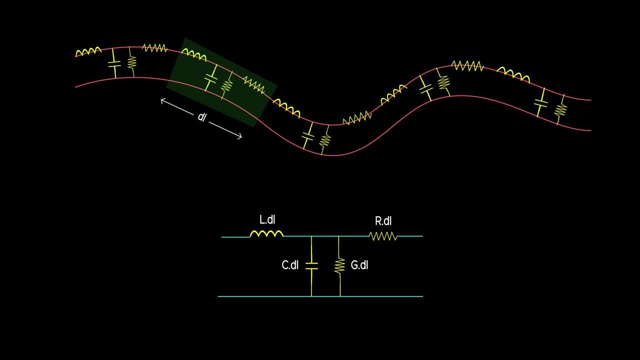 at each section. The analysis is very simple: Just applying voltage signal to the input of the section and measuring the change in voltage and current across the element. I'm not gonna bother you by the equations, but the final result is these forms: 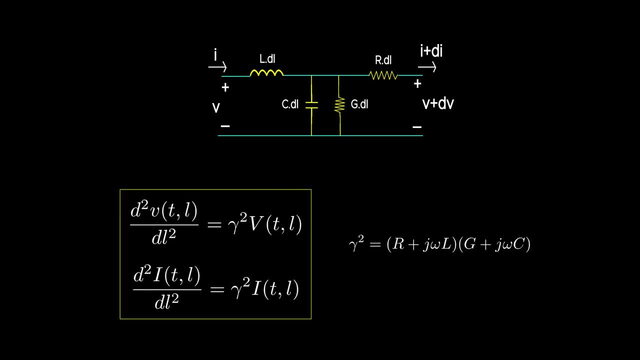 Voltage and current wave equations. where gamma is called propagation constant, a characteristic quantity of transmission lines, It depends only on the line parameters. Wave equations are simple differential equations telling us that at each point in time, each point in the line has different voltage and current based on its location. If we assume that the voltage and current varies sinusoidally, 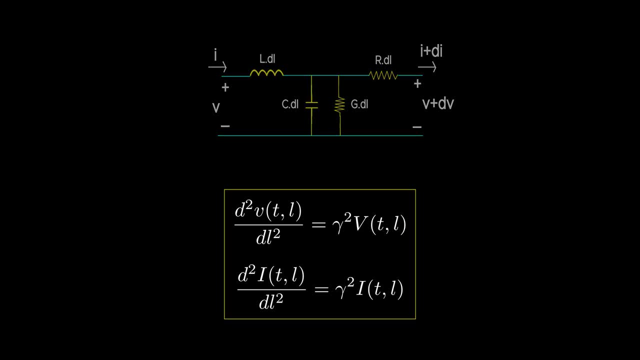 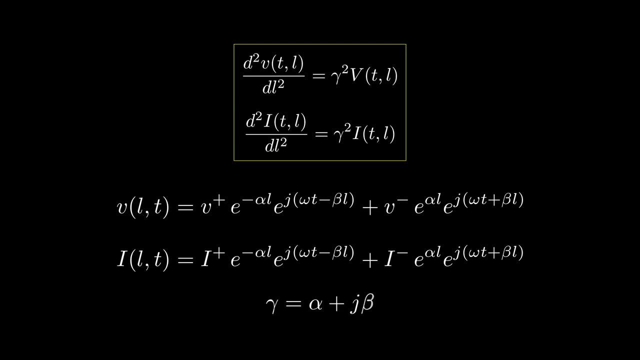 If we assume that the voltage and current varies sinusoidally with respect to time, the solution of the wave equations is consisting of forward traveling wave and backward traveling wave, where alpha and beta are the real and imaginary parts of gamma. Let's ignore the backward one. 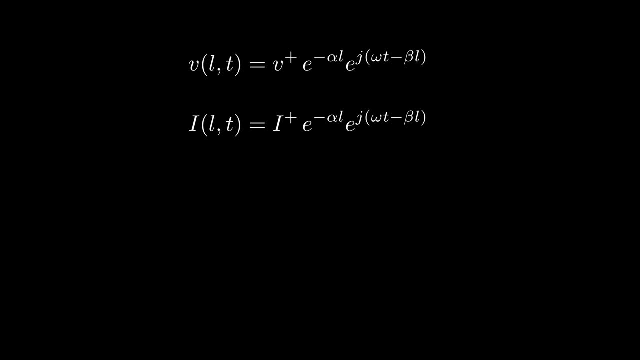 We gonna cover that in a separate video. when we talk about reflections Now, alpha represents the losses in the wire. Let's ignore it by ignoring R and G in each section to have a lossless line. Takin' the real part, we notice that the voltage and current varies sinusoidally with respect to time. 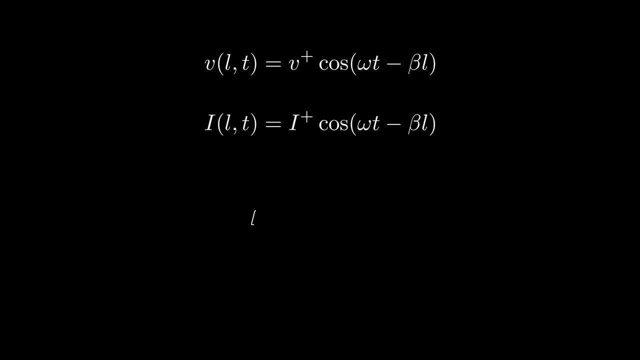 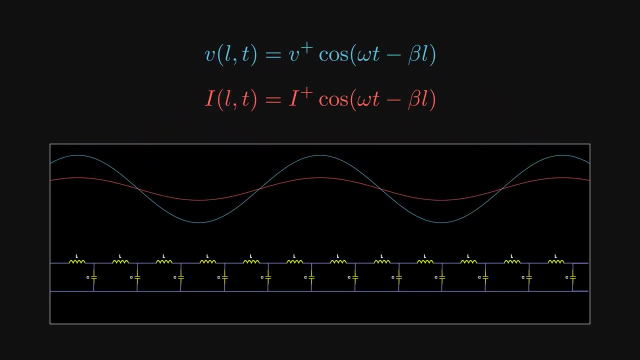 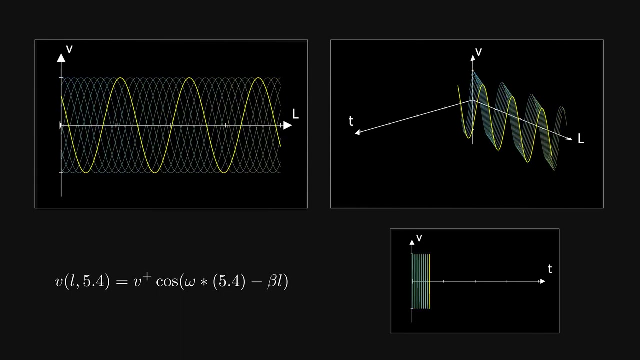 respect to time and distance along the wire. Notice that the current wave is a voltage wave divided by the characteristic impedance. At each instant of time, each point in the line has different voltage and current. By fixing the distance and varying the time, it feels like the signal is moving along the line. What we're doing here is just plotting. 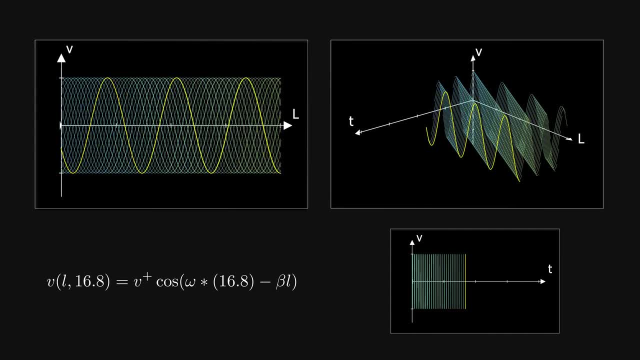 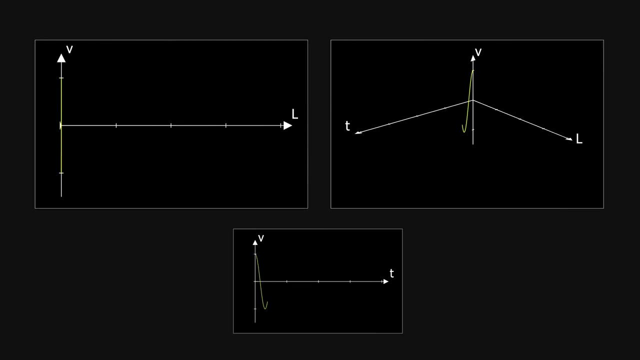 the voltage variation along the line as successive instants of time. Here we assume that the line is lossless, meaning there is no attenuation in the signal while traveling through the line. Voltage and current at each point in the line vary sinusoidally with respect to time. 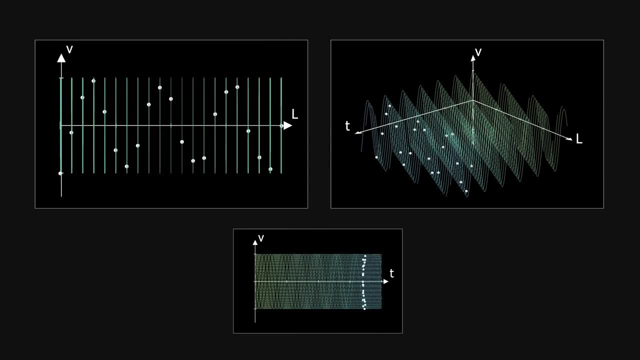 You can notice that by seeing the movement of the dot up and down or the height of each dot. it represents the voltage at that point in the line. Don't forget that the forward traveling current wave is just the voltage wave scaled by real 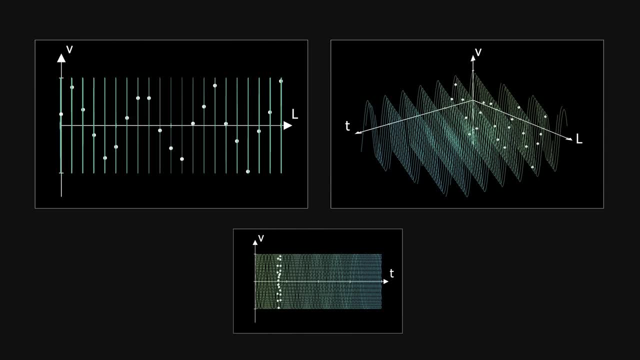 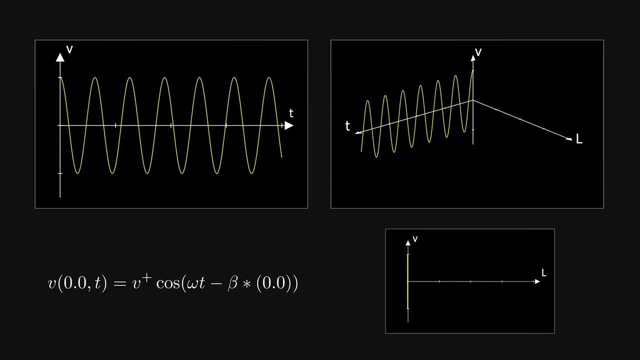 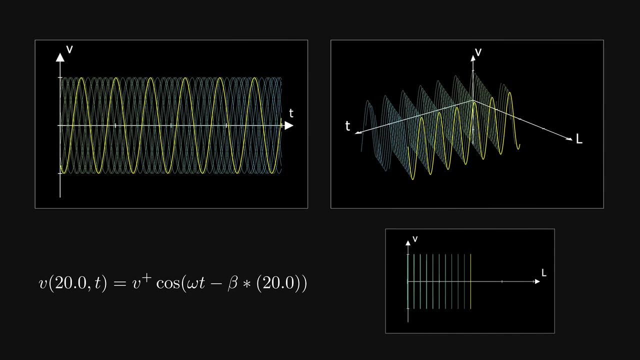 number the characteristic impedance, so it varies along the line the same way as the voltage. Notice that when we change the distance and fixing the time, it turns out that the signal is moving with respect to time, meaning for a lossless line. each point in the line sees a delayed version of the signal, depending on. 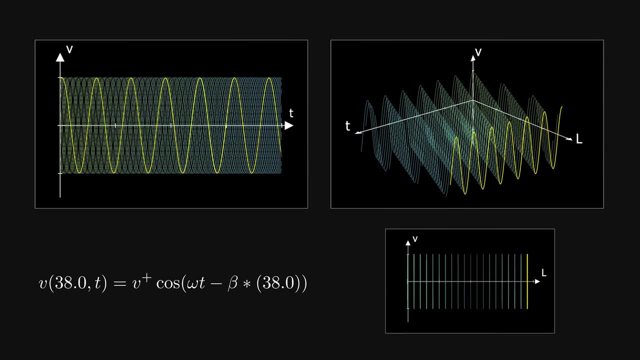 its location. The longer the distance from the generator, the higher the delay. That delay is a function of distance along the line and is linearly proportional to beta, the phase constant. If beta is equal to zero, there wouldn't be any delay along the line. 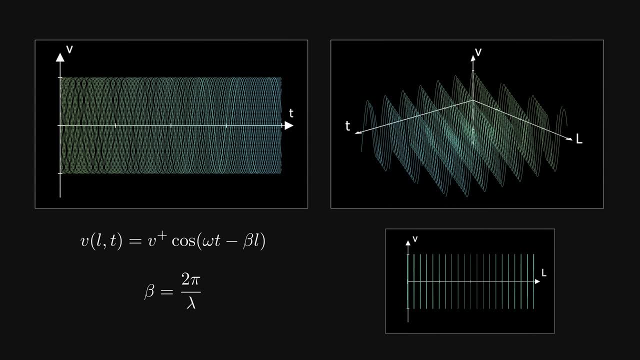 Beta is equal to 2 pi over the wavelength. That confirms that the larger the wavelength of the signal, the less would be the delay. In the next video we will use the simulator to get more insight inside of what happening inside the transmission line itself.